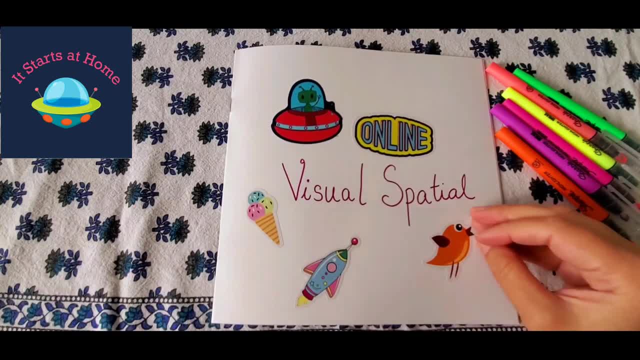 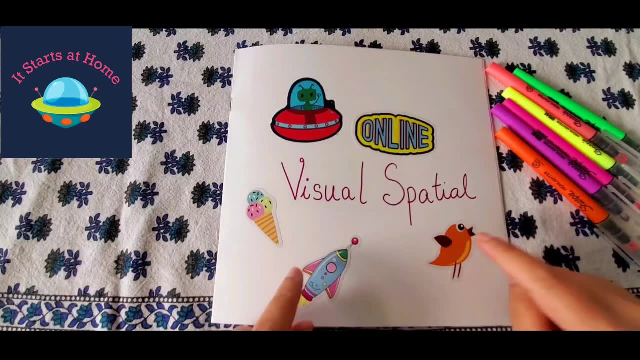 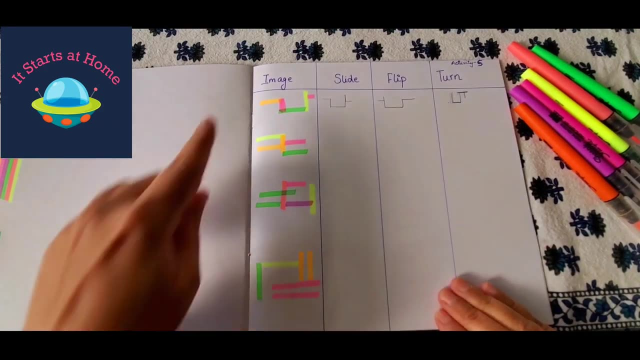 teaser and visual spatial activity for, I would say, kids up six to nine, or you could modify them for kids four, and I would exactly tell you how you can modify that too. Okay, so let's get going. Okay, so this is the image. Okay, this is how you're going to slide, flip and turn. So you have. 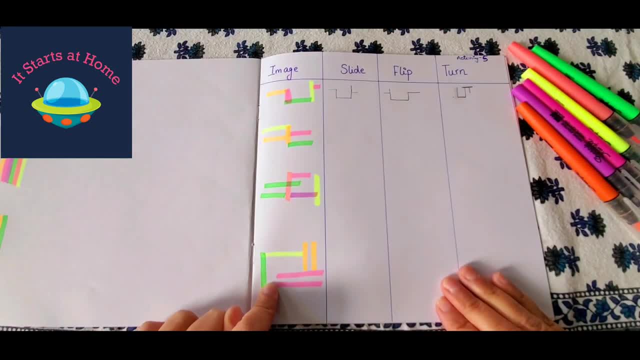 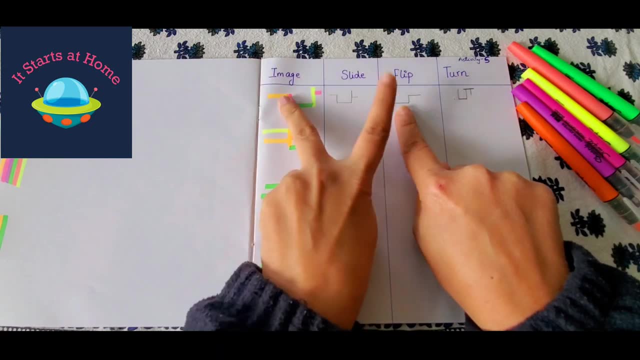 one, two, three, four. There are four of them. So you're going to slide, flip and turn, So you have four different designs that I've made here. Slide means you copy exactly the same design. Flip is something that you reverse. Okay, so if this is like this, you make it like this in turn, and this: 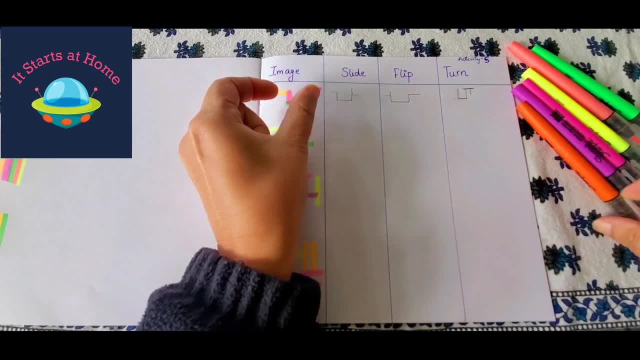 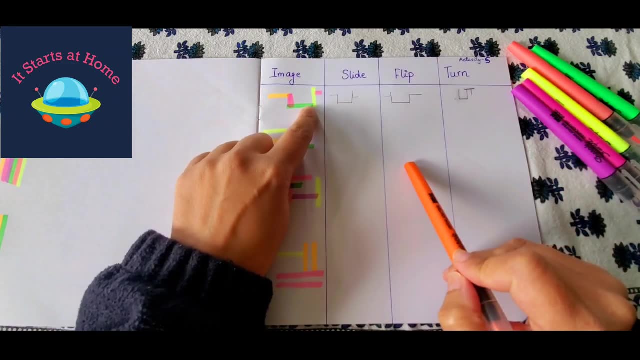 is called turn, and in turn you take a picture, So like if the pen is like this, you turn it like this. Okay, so here, all these shapes, or all these lines that you see, have been turned around to this shape. So this was activity number five, but just to show you how you can make it like this. So 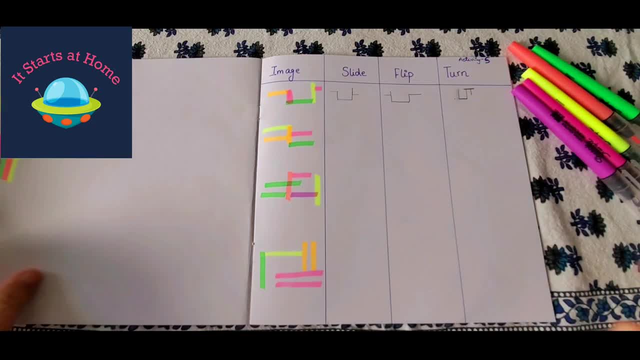 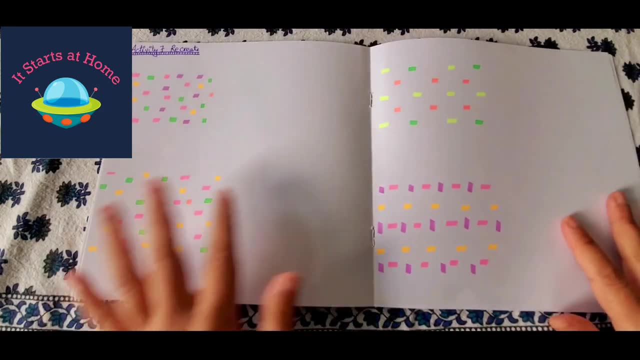 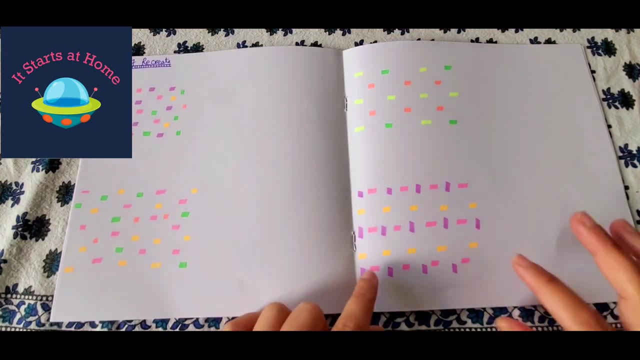 just giving you an idea how exactly all of them will be done. Okay, let me share with you another one, which is my activity number seven. So you have a pattern which is going on here. Okay, for these four designs, and the kids have to recreate. and when I say recreate, they have to make it. 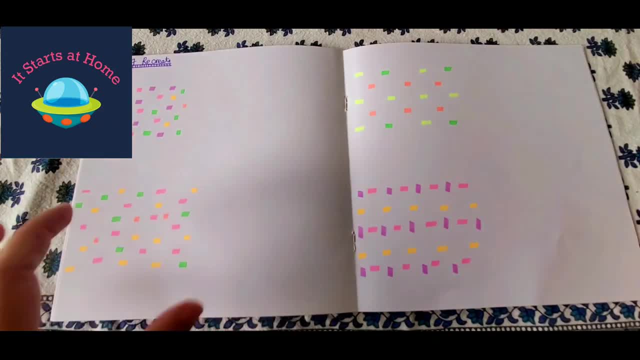 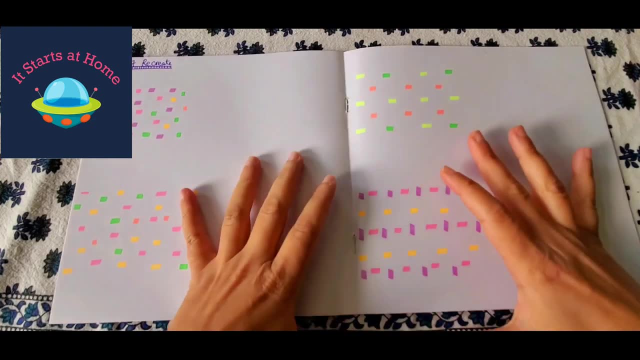 exactly the same the way they are. Definitely the positioning can be here and there, but like if there's a purple and pink, purple and pink, purple and pink, the way they are, once they start doing it, they will see a pattern and that's what I'm going to show you. So let's go ahead and 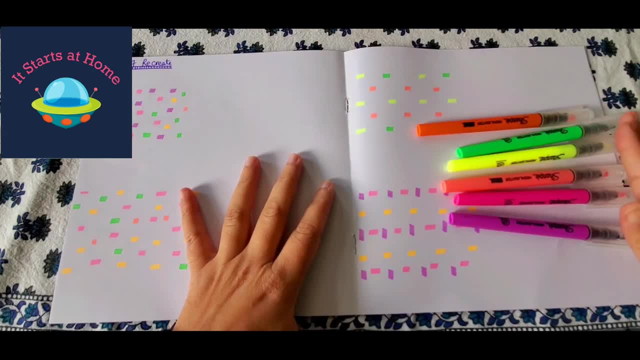 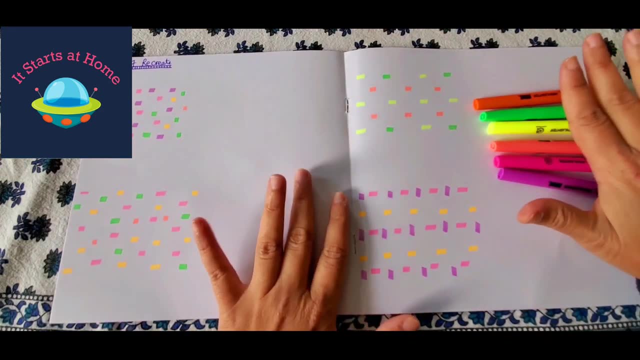 take a look. Okay, so this is activity number eight. So this is activity number eight. So that's how the colors that you've used- like if I have used these six highlighters, you could use any six sketch pens. Make sure the kids have to use the same, So just keep them next to them. 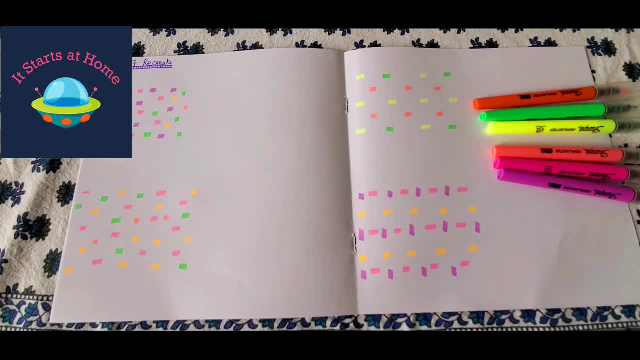 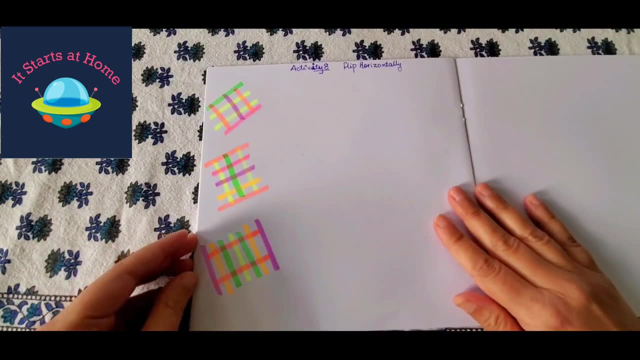 That's all. That's the only thing that you need to finish this activity, Nothing else. So they're recreated and there are four different designs that they can do. Okay, let me show you another one. So this is activity eight and this is flip horizontally. Okay, so there are these three. 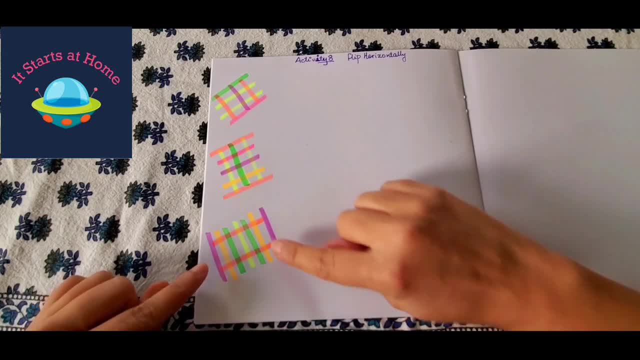 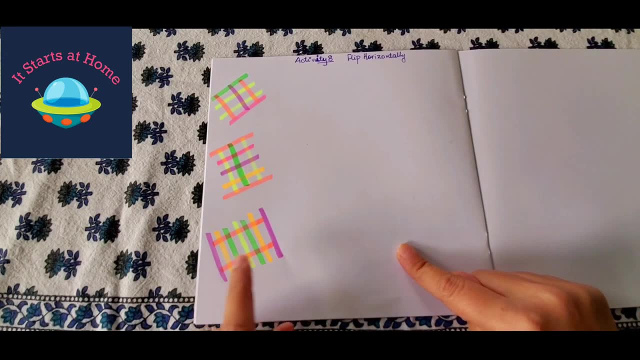 designs, The way they have been made, are you know they're going to be like this. So you have two purple lines. Okay, there are horizontal and vertical lines that are going and the kid needs to flip horizontally and recreate the same design right here. Okay, so using the same pens. 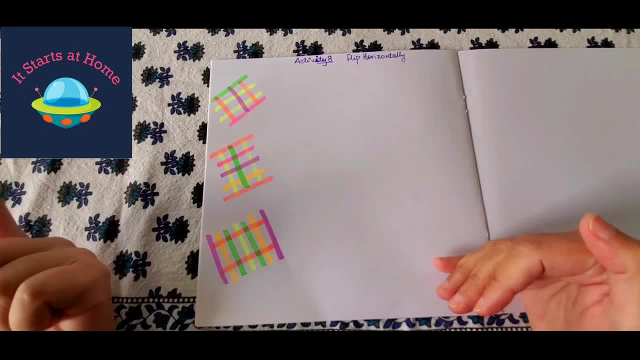 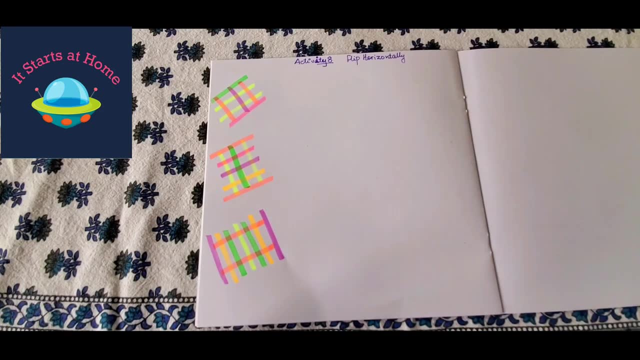 looking at this. So by now your kid needs to know what is flip, horizontal and vertical. They need to know what is a mirror image. So with these activities it's just so much of brain teaser that you might think in the beginning that it's too easy. But trust me when you have. 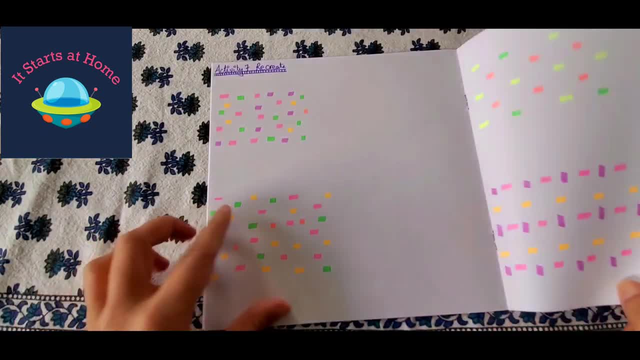 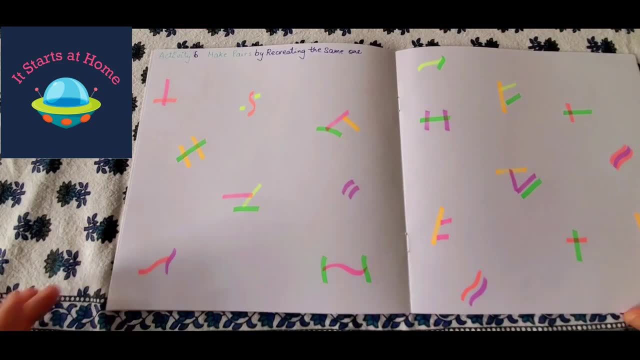 so many colors going on. you need to flip horizontally All these shapes and all these elements. do not make it very easy. Okay, let me make you see activity number six. And in activity number six you would see there are so many gathered, different designs and patterns. Each one 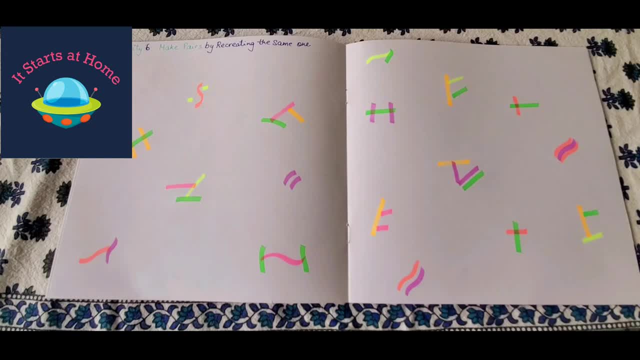 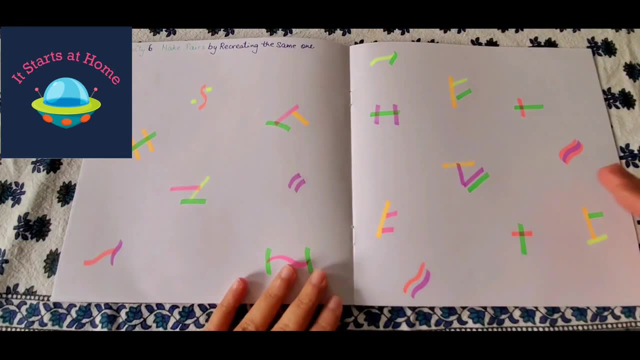 of them are different for one another and they all have different colors. Okay, so what you have to do is you have to make pairs by recreating the same one, Because we are doing it for the older group, so they don't have to do the matching, because matching is super easy. But if you do it for the 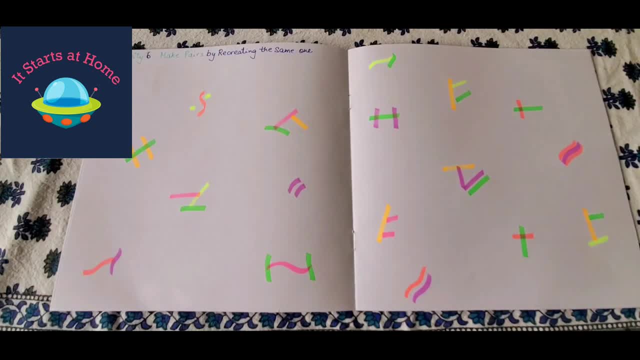 older group. you can definitely make matching. But, guys, if you try this activity, make sure that you share it with me. or if you tag me, if you share it on your social media, make sure that you just tag me there and it starts at home. or Sonali Kapoor, I would be happy to see your version. 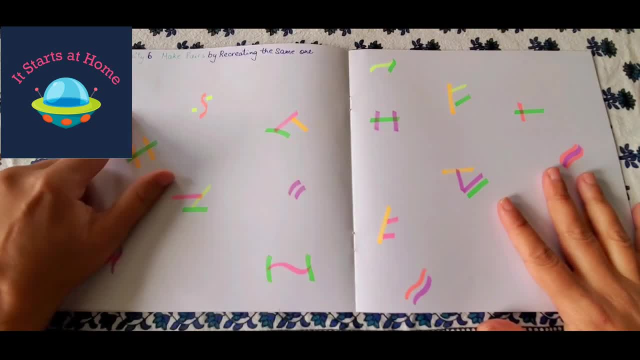 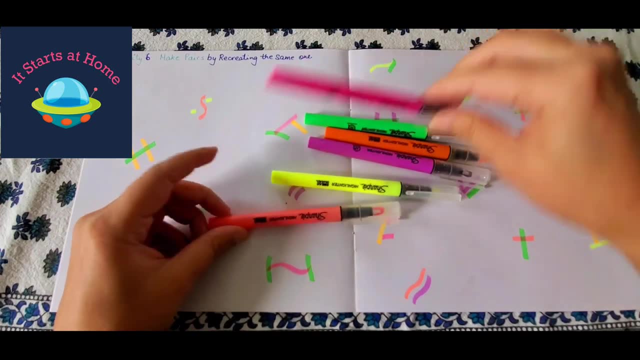 Okay, so the elder kids have to recreate the same. So if this is one of the shapes they have to figure it out, what colors would they need? Okay, and I have used two similar colors, So these are the ones, And then he needs to recreate the same one right here. So you have ample of space, just 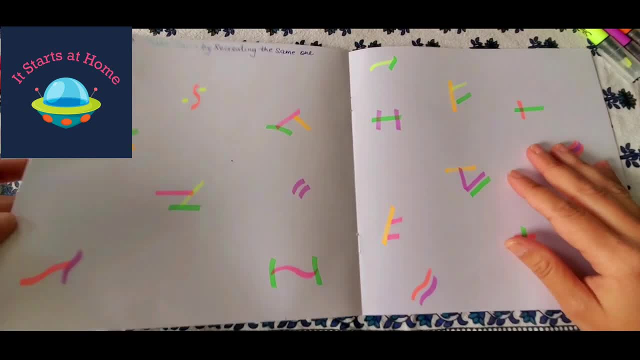 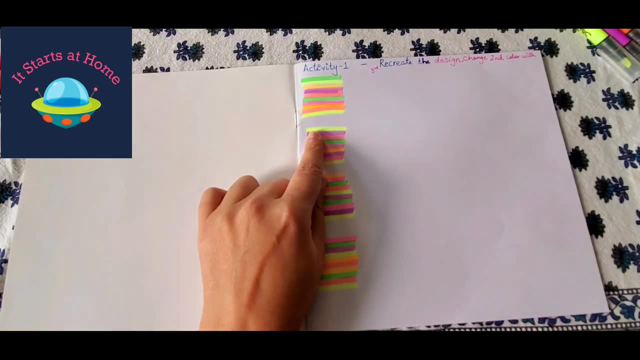 on the other side. So you have ample of space just on the other side. So you have ample of space all along to create the same ones. Okay, let me go with the. let's go with the first activity. Okay, so this is recreate this, sorry, recreate the design. change second color with third. Okay, 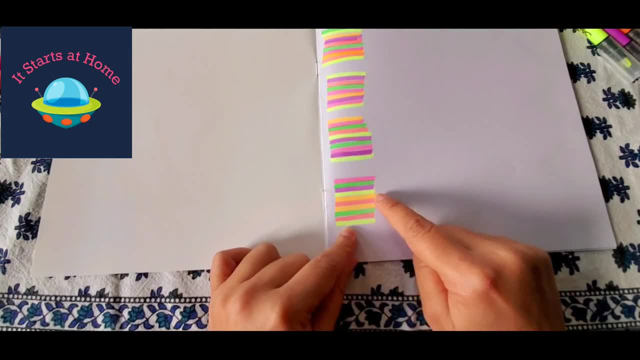 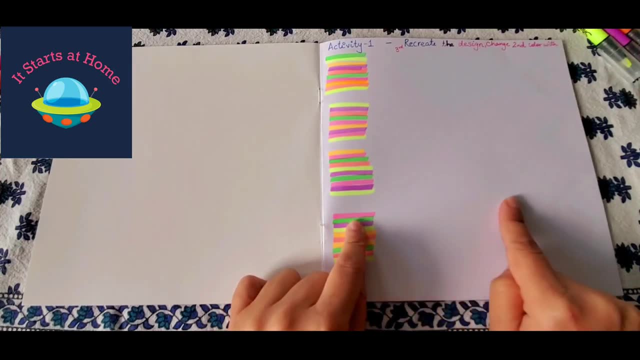 so let me take an example of this one. So you have 1,, 2,, 3,, 4,, 5,, 6,, 7,, 8,, 9,, 10.. You have 10 here. Now they have said you have to change the second color with third. So when you're making 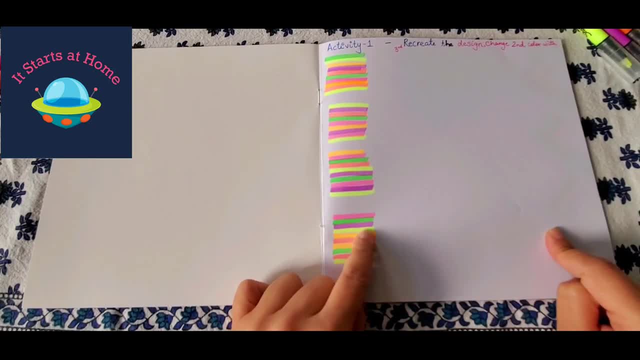 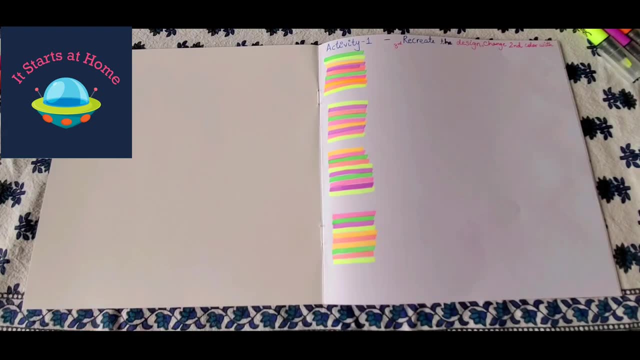 this: you have to go pink and purple, Okay, and then green And then the following color. So you have to recreate, but you have to make sure that you're changing, Okay, and if you have to make it more difficult, which I think I would-